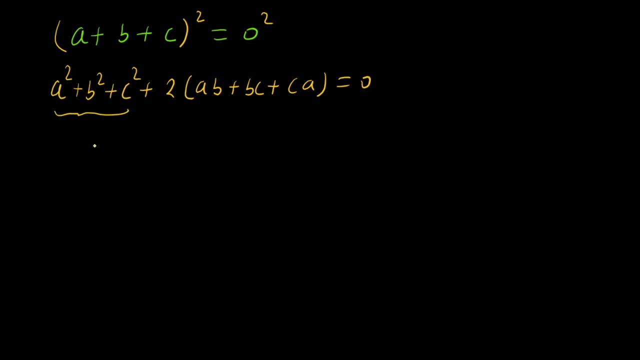 And we know that value of a square plus b square plus c square is 434 plus 2 times ab plus bc plus ca, and this is equals to 0.. Now if we subtract both side 434, then here in left hand side this is cancel out- then 2 times ab plus bc. 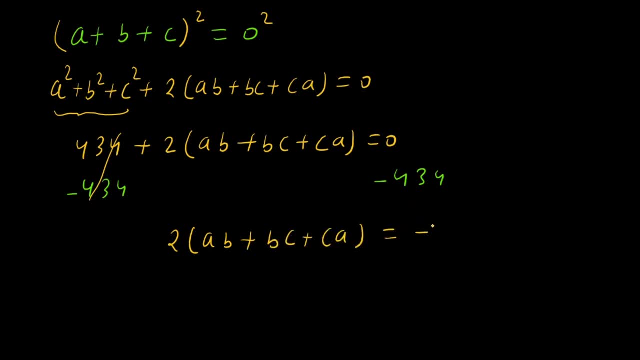 Plus ca, and this is equals to: in right hand side we have 434. now if we divide both side 2, then in left hand side this 2 and this 2 is cancel out, then ab plus bc plus ca and this is equals to minus 217.. 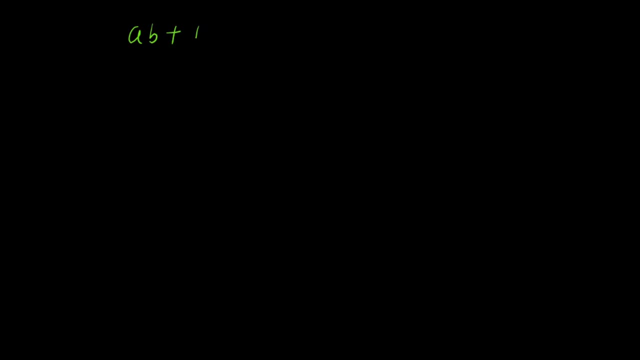 Here ab plus bc plus ca. this is equals to minus 217.. If we take square both side, we know that value of a square plus bc plus ca is 434.. If we take square again both side, then in left hand side we will apply this identity: x plus y plus z, whole square. this is equals to x square plus y square plus z square plus 2 times xy plus yz plus zx. 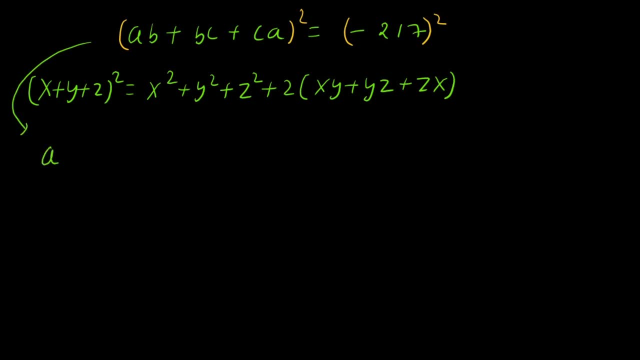 Then, in left hand side, a square b square plus b square c square Plus c square, a square plus 2 times ab times bc plus bc times ca plus ca times ab, and this is equals to minus 217 square, that is 47089.. In left hand side, a square plus bc plus ca times ab, and this is equals to minus 217 square, that is 47089.. 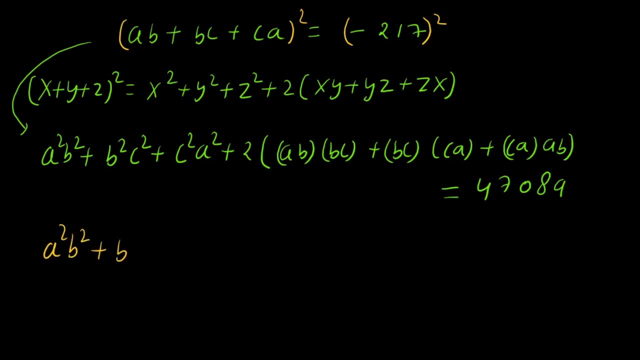 A square b square plus b square c square plus c square a square plus here 2 times. this is ab square c plus b times c times c times a. that is b times c. square a plus c times a is multiplied by a times b, Then c times a square b, and this is equals to 47089..